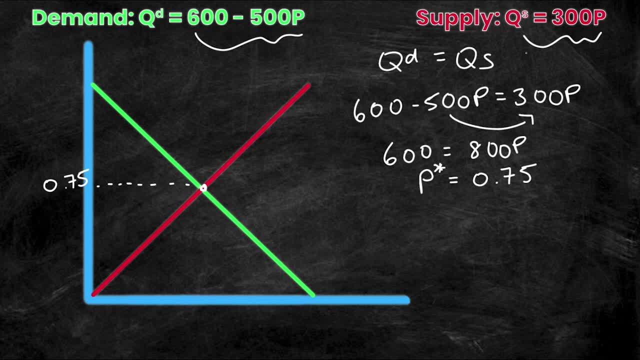 this P star and to sub it into either the QS or QD equations, and I know that they're both going to give me the exact same Q value and that will actually be my Q star. So I'm going to sub it into QS, as that's significantly easier, and we'll do that right. 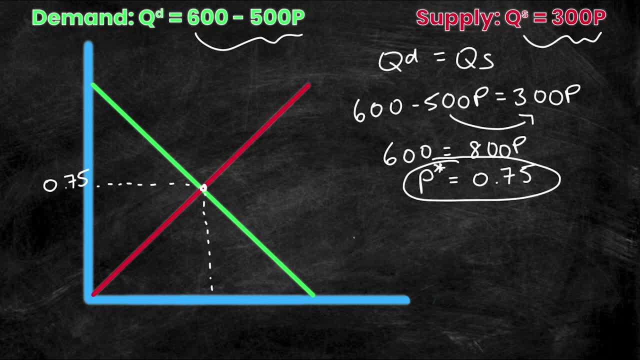 now. So my P star value is right here and we'll sub into QS for my Q star value. So Q star is simply equal to 300 times P, and I know that P is 0.75.. Therefore, Q star is equal to 225.. 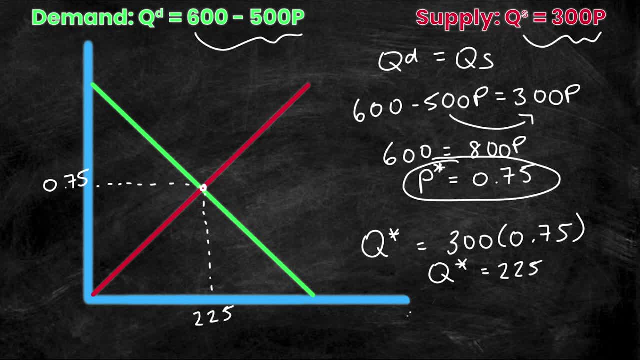 And so now I have my labeled graph. Don't forget, of course, to label your axes. So Q and P. Now I've got my labeled equilibrium, which is a price of 0.75 and a quantity of 225.. But now we're going to look at two scenarios: a shortage and a. 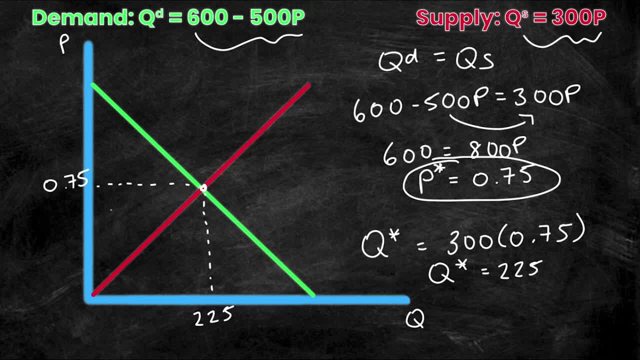 surplus, And we're going to take a look at what that means for the supply and demand graph. We'll start by looking at a surplus. Let's say that for some reason, instead of being 0.75, the price was actually set at approximately 0.75.. So we're going to take a look at what that means for the supply. 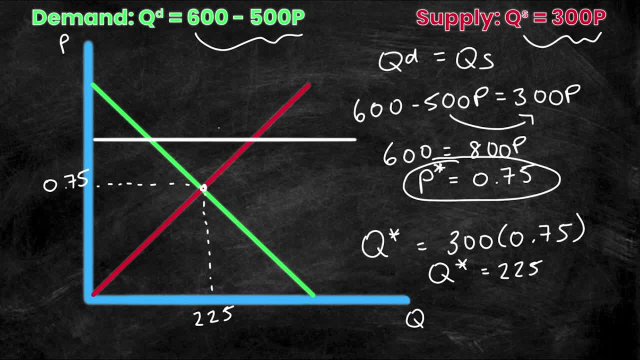 and demand graph And we're going to take a look at what that means for the supply and demand graph. So we'll have this line right here: represent the new price, and it'll be at 1.00 or $1.. Well, now we don't have an equilibrium point, but we actually have two different intersection points. 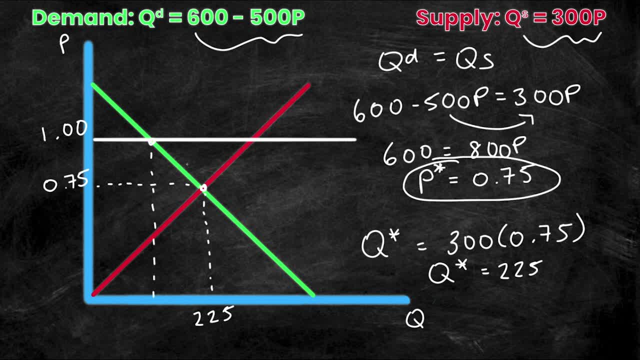 right here where the new price intersects the demand curve, And over here as well, where the new price intersects the supply curve, And these are not at equilibrium. So how do we calculate these two quantities? Well, we actually have to sub in $1.. 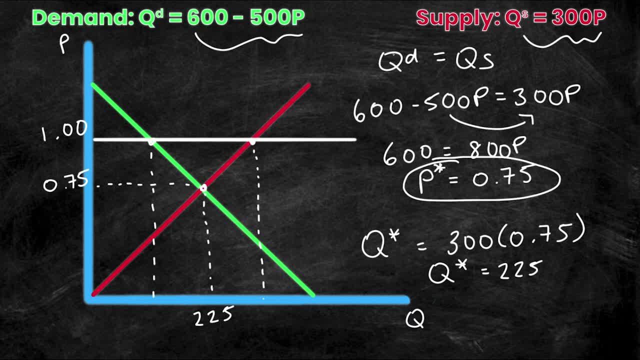 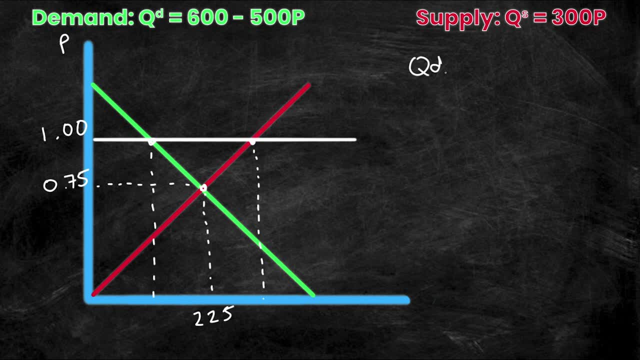 into both the Qd and Qs equations separately. So let's do that. So first let's sub it in to the Qd equation. So Qd is equal to 600 minus 500 times the price. Well, this new price is actually 1.. So Qd? 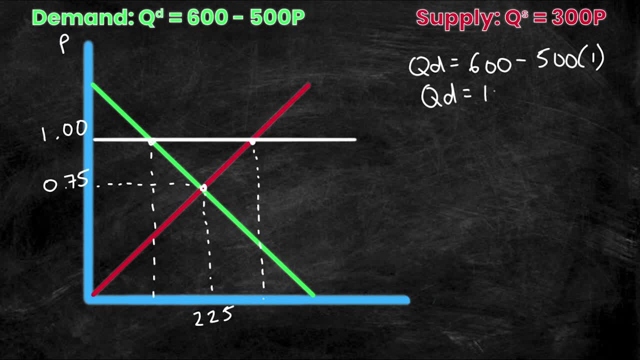 is going to be 600 minus 500, which is 100.. So this value right here is equal to 100.. Now let's do the same thing for Qs. So Qs is simply equal to 300 times P. Well, P is just 1.. So Qs is equal to 300. 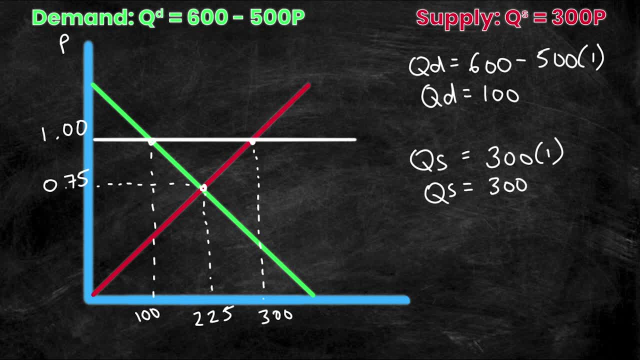 Now what do we notice about this? Well, we notice that Qd is strictly less than Q star. That is, in this scenario, we have a surplus and Qd is 100 and Q star is 225.. So it's an obvious statement that 100 is less than 225.. Therefore, in this scenario, 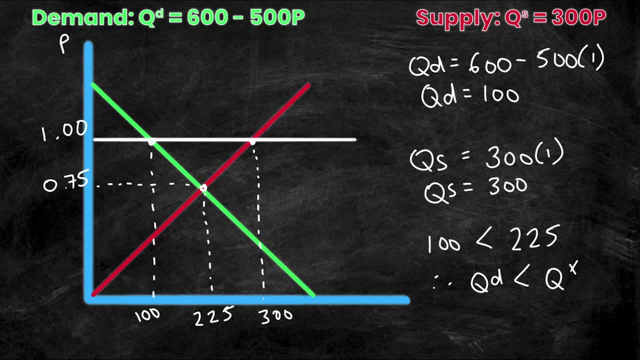 Qd is less than Q star. At the same time, we notice that 300 is greater than 225. Therefore, Qs is greater than Q star. Now does this logically make any sense? Well, it does. Via the law of demand, you would expect that if the price goes up, demand for the good goes down. 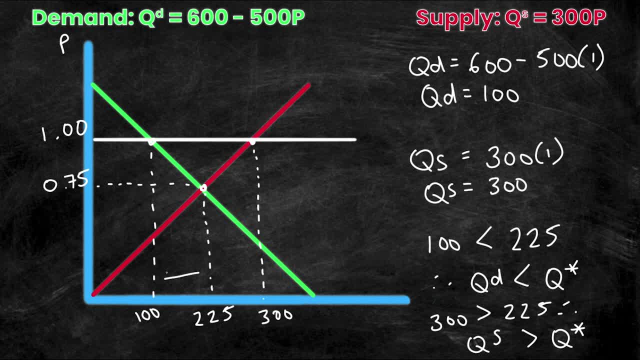 So we actually see a decrease in demand by this amount here minus 100, so a decrease in demand by 125 units. At the same time, an increase in the price due to the law of supply would assume that supply increases. So we see that an increase in supply. 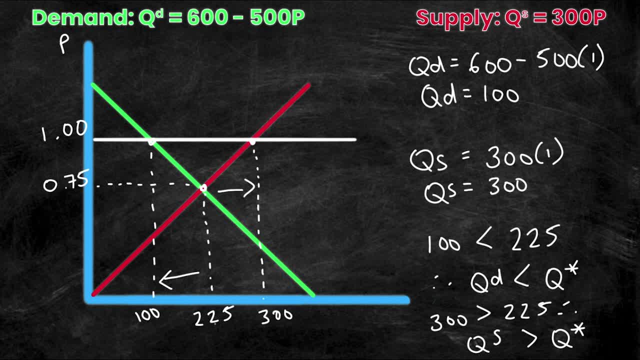 happens by this amount here, the difference between 300 and 225, which is 75.. So there's two different effects happening, and that does make sense, via the law of demand and the law of supply. So in this case demand is really low, It's at 100, and supply is really high, It's at 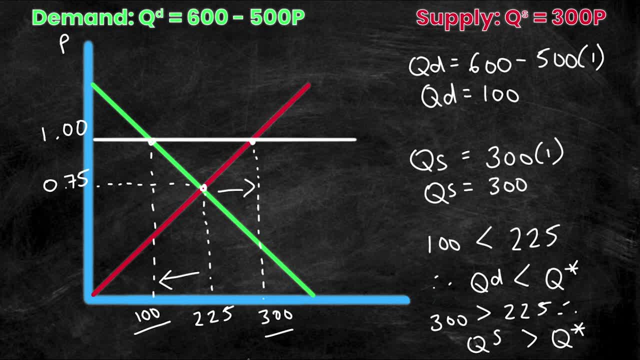 300.. So we have way more products being supplied in the market than there is a demand for, and we would call this a surplus, meaning that there's more supply in the market than demand. And you might be wondering, well, how much actually gets traded in the market then? Well, at a price of 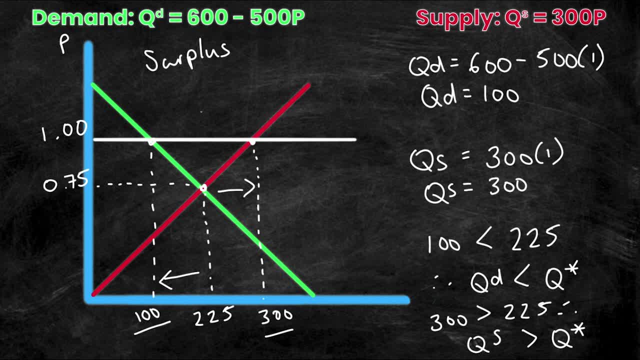 $1,, you will always trade at what we call the short side of the market. So if you're working your way from left to right, it will always be the first intersection point with the price, which actually happens to be at. Q equals 100,, which means that in this market, 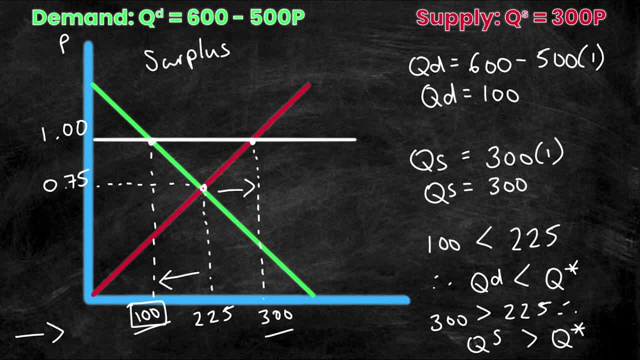 at a price of $1, only 100 units will be traded in the market, Even though there's an additional 200 units being made available. the difference between 300 and 100, even though there's an additional 200 units available, because there's no demand for them, they won't actually be sold. 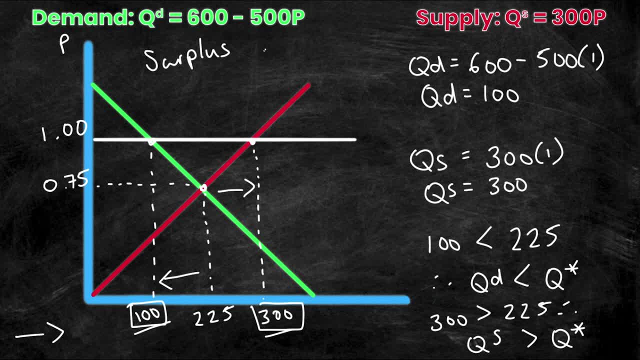 At a price point of $1.. So there's a surplus of 200 units in the market, And that's simply the difference between how much is supplied and how much is actually demanded. So 100 units will be traded in the market. Even though there's 300 units available, there's only demand for 100. 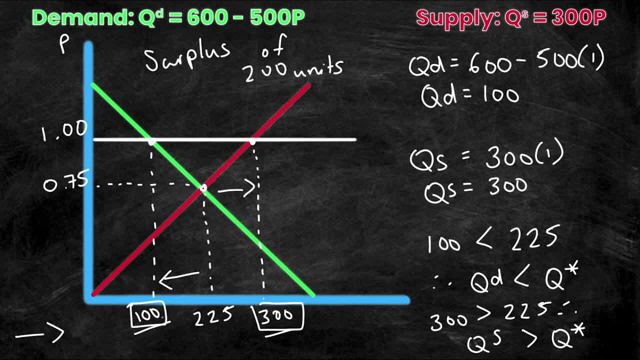 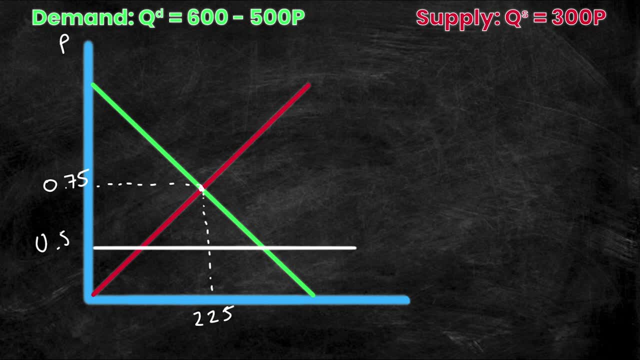 units. Now let's take a look at what happens when there's a shortage. Now let's say that the price is actually something lower. Let's say 50 cents or 0.5.. Well, we're going to do the same thing that we did before: We're going to sub this new price. 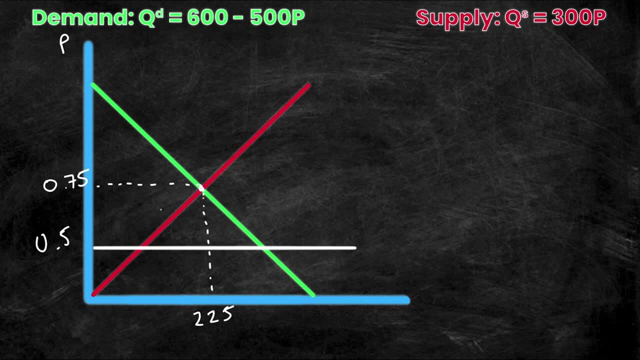 this one down here into both the QD and the QS equations and we'll see where these two intersections are made. So if we sub this into QD, then we get 600 minus 500 times 0.5, which is 600 minus 250. 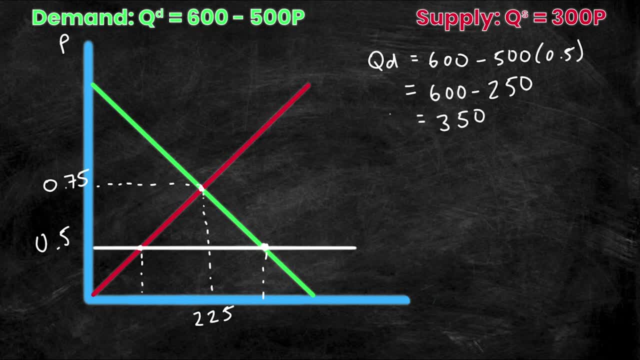 which is equal to 350.. So where the demand curve intersects, this price line is at 350 units over here. On the contrary, QS. let's sub it into this equation. see what happens: 300 times P, which is 0.5.. And this is simply equal to 150, which is over here somewhere. So now the reverse. 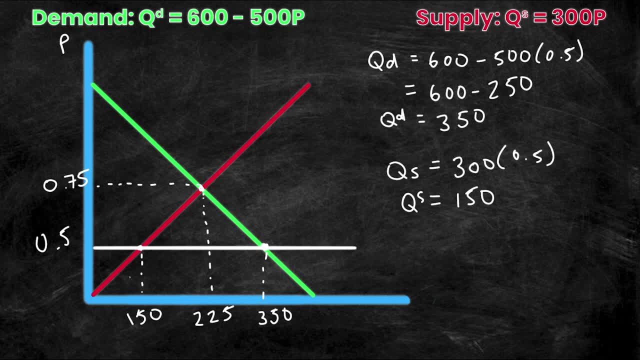 is true. We're actually seeing a shortage in the market, And you can see this, as QS is strictly less than QD. 150 is less than 350.. And so, therefore, even though there's a demand at a price of 50 cents, even though there's a demand of 350 units, 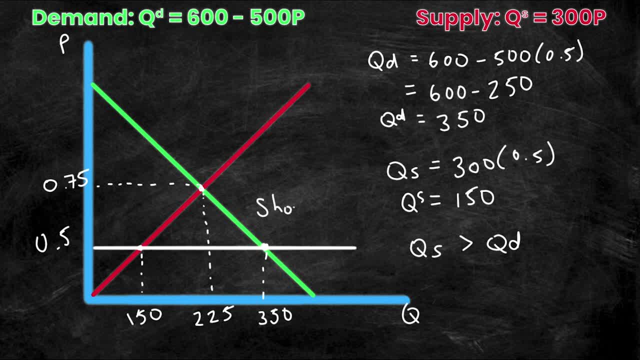 there's only 150 units available in the market, So there's actually a shortage. Well, how do you know how much the shortage is? Well, if you look at the price of QS, you can see that QS is less than 350 units. 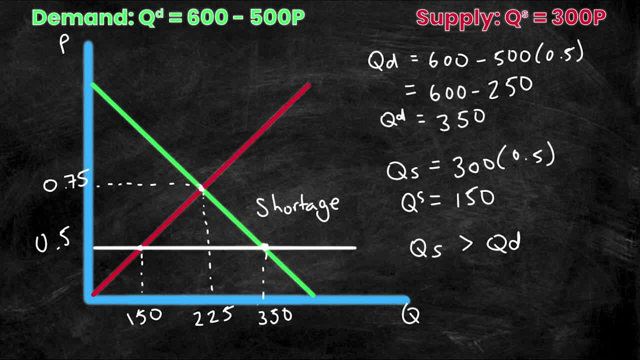 So there's actually a shortage. Well, how do you know how much the shortage is? Well, how do you know how much the shortage is? We just take the difference in demand and supply, So we know that the demand is 350 units. So that's.